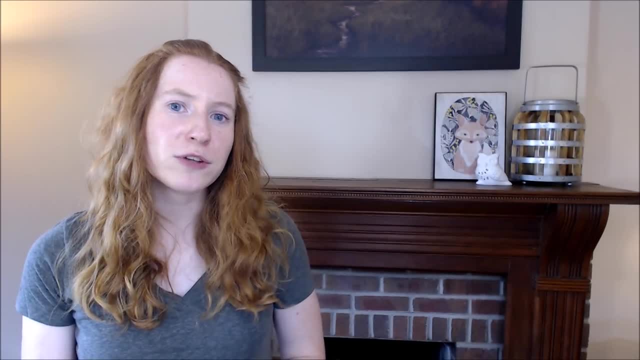 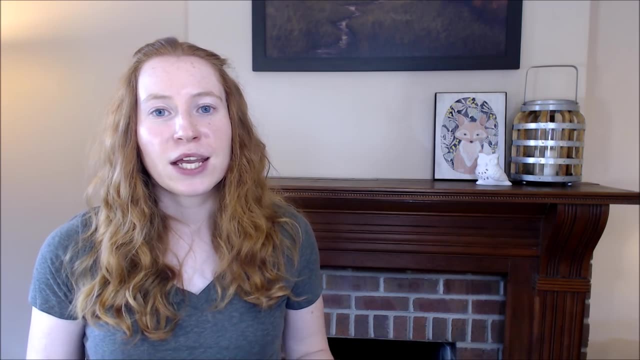 you hear the writing advice that you should write realistic characters. We all see characters that are clearly not realistic. They have skills that don't exist in reality. They have outlandish personality traits and it can be hard to understand. in what sense does the character 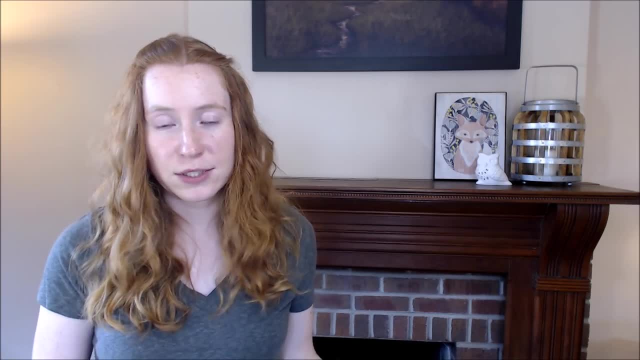 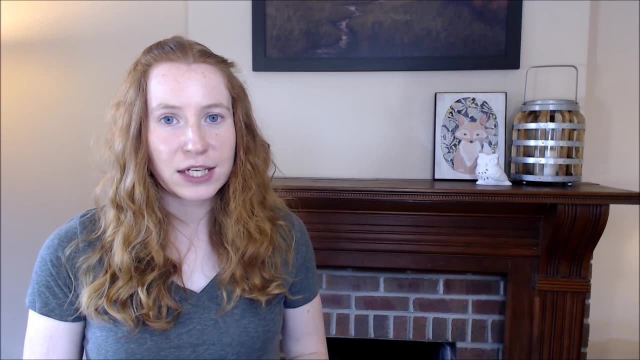 need to be realistic. when you see all these characters that just don't seem realistic at all. But the key to creating a realistic character is not necessarily to create a character that feels as if they exist in reality, but rather to create a character that makes sense within. 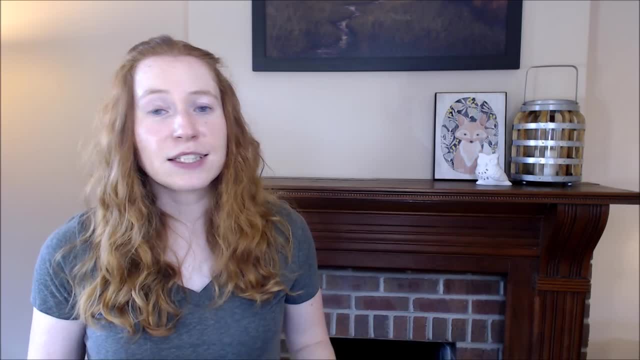 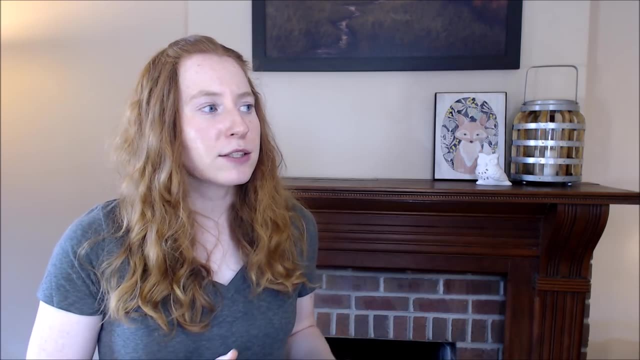 the context of your book. So if you're writing a fantasy and it's very outlandish and unrealistic and it's just a wild story, there are still characters that are realistic. There are characters that will feel as if they make sense existing in this world and then 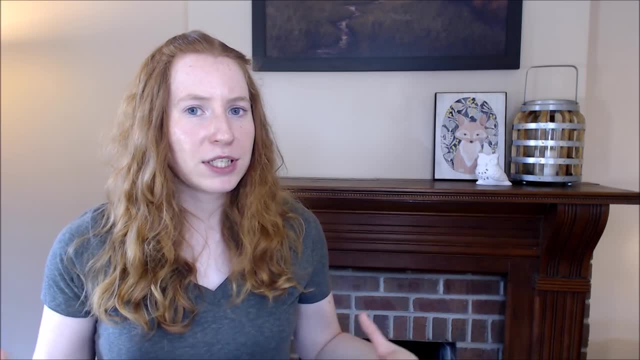 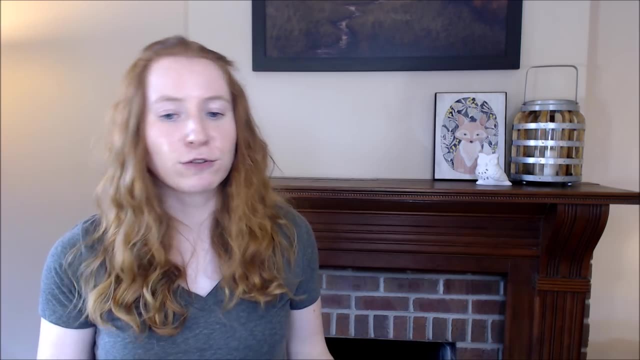 characters that just don't quite feel right. So when we're talking about realistic characters, we're talking about a character that makes sense both within themselves. their motivations, their flaw, their backstory all work together. it all makes logical sense, as well as their 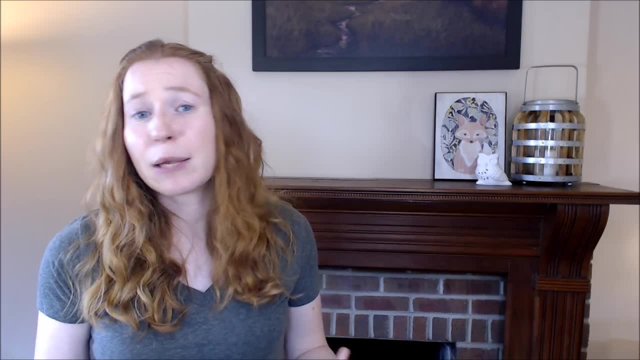 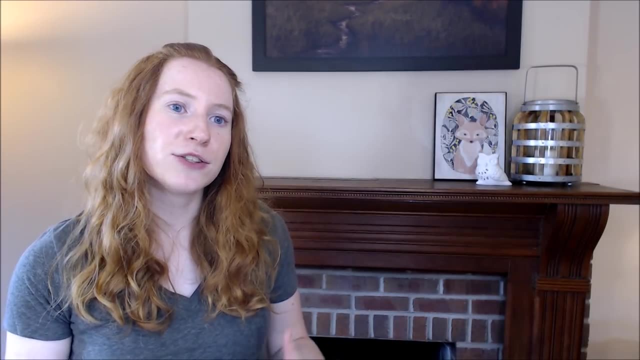 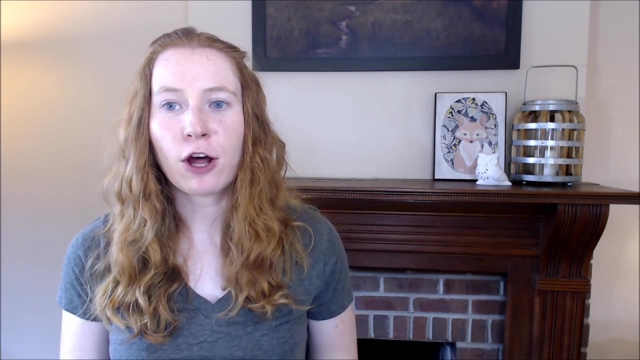 personality traits being logical, making sense, being possible in the context of the novel. And then also we're talking about how suited the character is to the story, to the setting, to the plot. How well does this character fit in? We've already talked a lot about motivation and flaw and backstory and things like that. 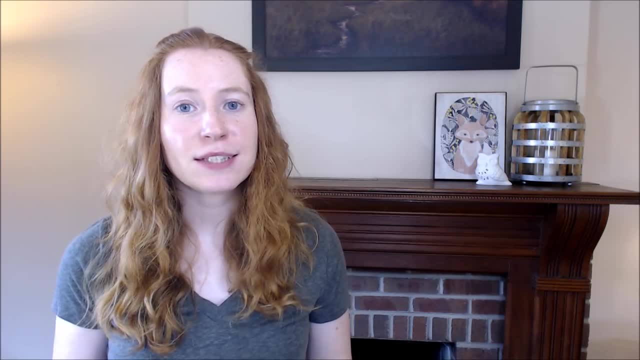 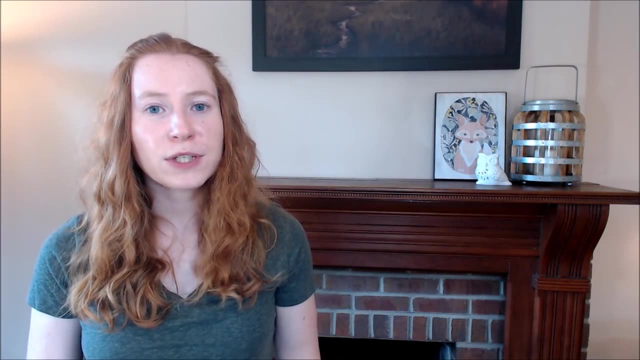 so today I'm going to try to focus more on character traits and why certain traits might feel realistic or unrealistic in the context of your novel. You'll know if your character isn't feeling realistic because agents and editors will probably tell you that they don't connect. 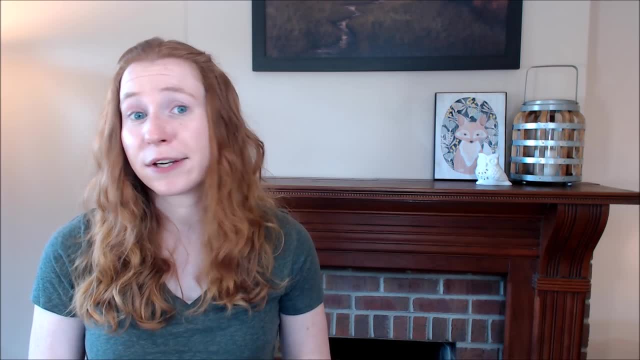 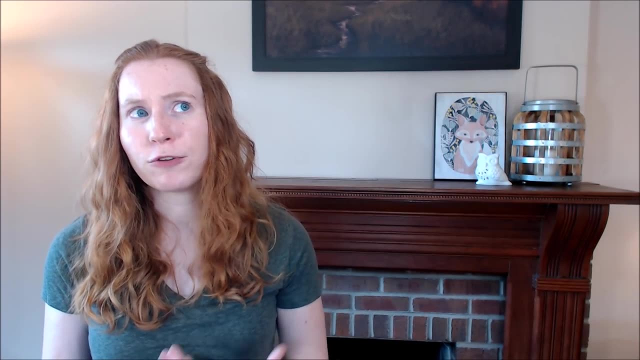 with your character and beta readers might tell you that they find your character annoying or unlikable. This normally doesn't come from negative traits. it normally comes from an overabundance of positive traits. The character just feels too well suited to their environment. 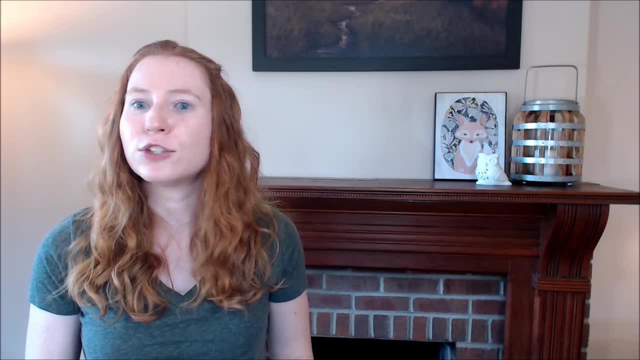 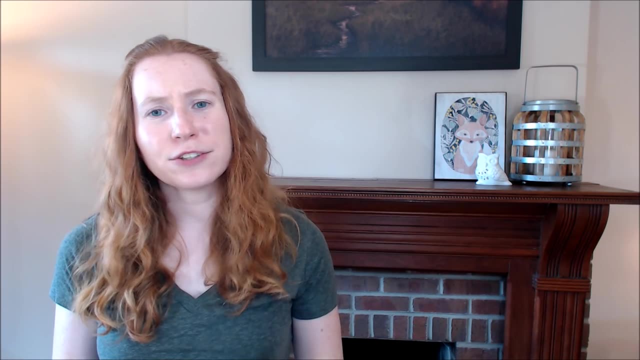 they're too capable, they're too perfect, they make friends too easily. things just work out too well and too nicely. So I'm going to list out some traits that are very common in characters that are considered to be unrealistic or unlikable. It's important to note that these traits aren't 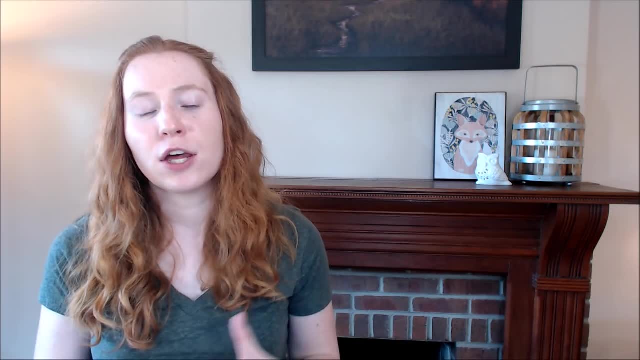 bad inherently. It's just a matter of how well they fit in the context of your novel. So if you're writing a novel and you're writing about a character that you don't like, it's okay to use them in your characters. The problem occurs when the traits aren't included for any real reason. 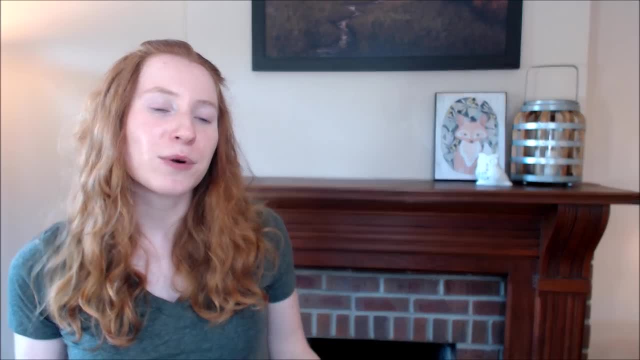 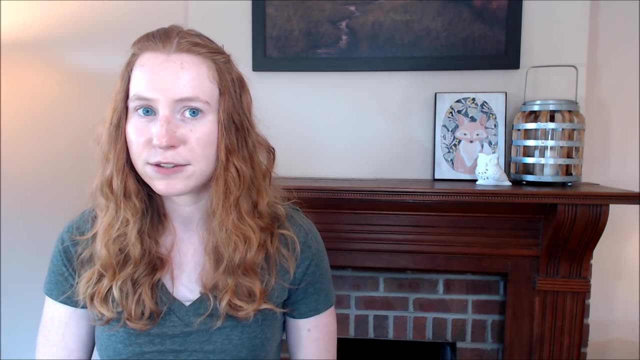 and they're sort of thrown in to make the character just seem better or to create sort of a fantasy life or a fantasy character. So the first type of trait that might cause you some trouble is physical appearance. It's very common for writers to create characters that are unrealistically. 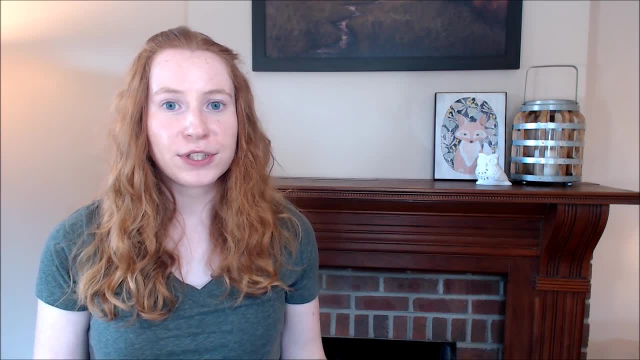 beautiful or handsome, and they may even have alternative appearances or something unusual about their appearance to further enhance their character. So if you're writing about a character that you don't like, it's okay to use physical appearances as well. You might even be writing about 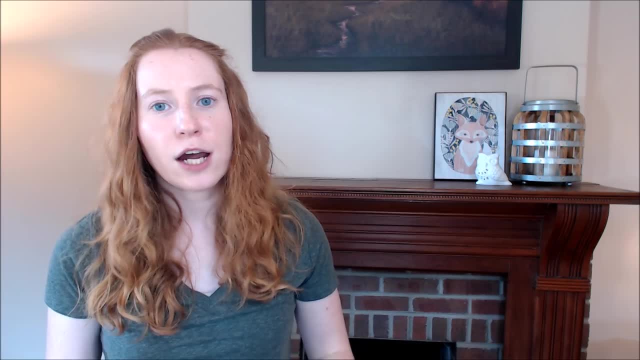 a character that's just a little bit more of a character than the real character, or a character that's a little bit more of a character, or a character that's a little bit more of a human, And it's important to note that physical appearances. you do see some of these traits. 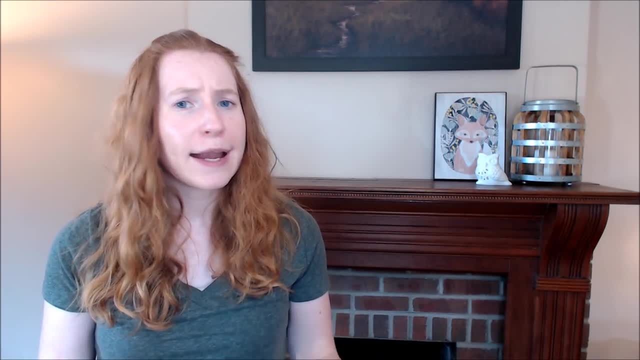 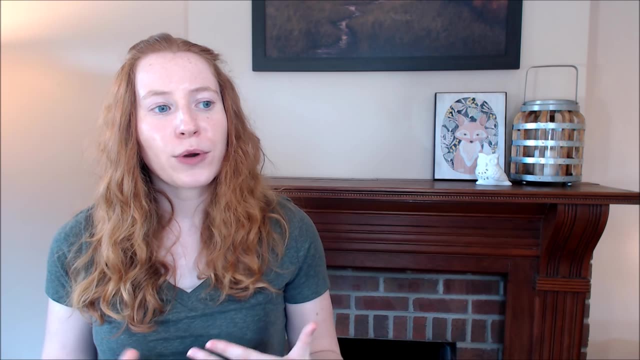 in a lot of your characters that you can tell them to be very unique. So there are ways in which you can draw a character that's more unique, but then you have to consider the traits that they have and why they're unique. So this might be an unusual or non-existent hair color or a high 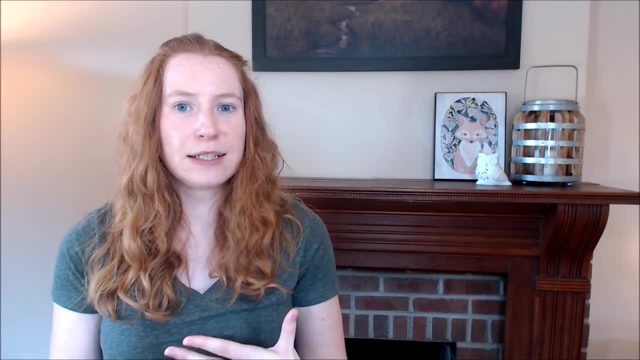 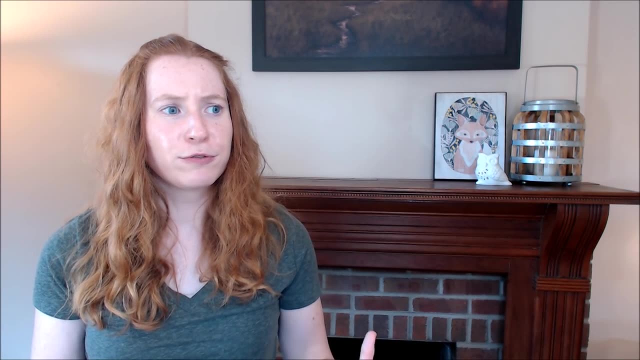 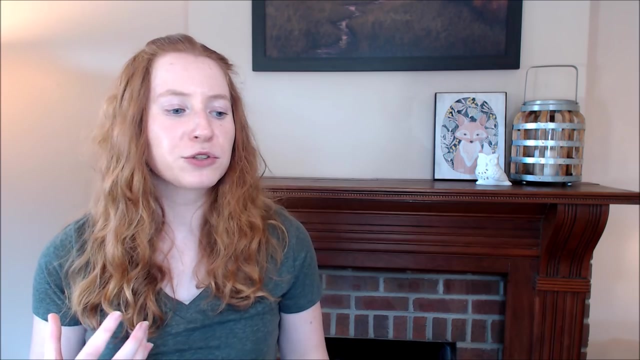 aura around the character, a sort of sense that this character is unnaturally mesmerizing. a lot of the time unpublished manuscripts will include this sort of factor of people are just attracted to the character and it's sort of not explained, Or it may be mentioned. the character is 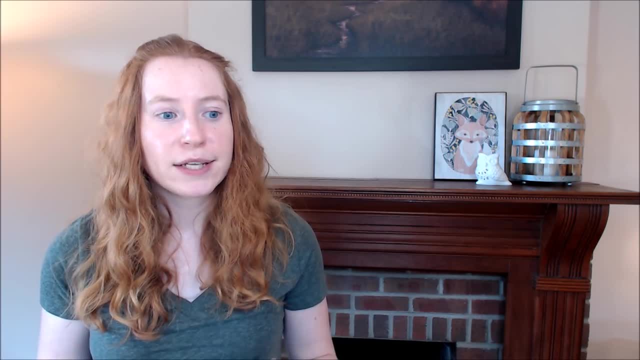 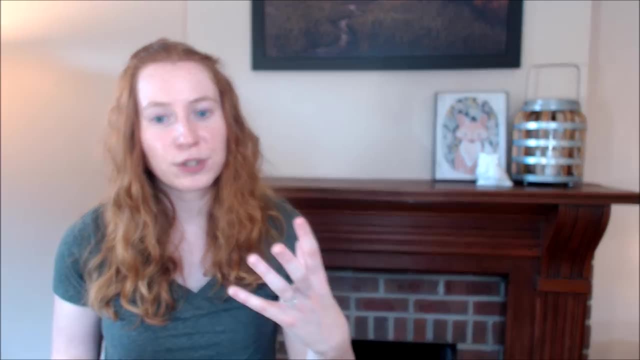 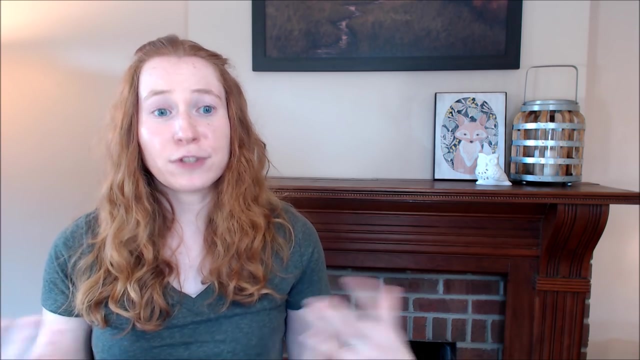 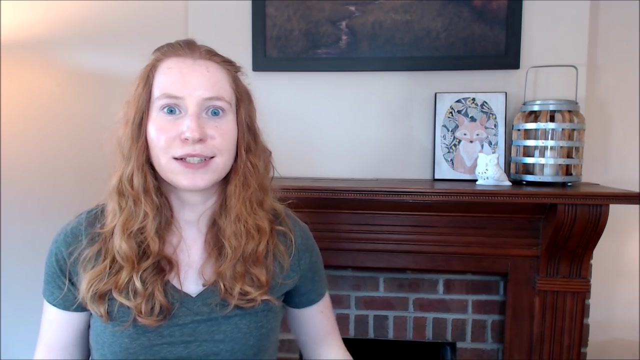 normal looking or plain looking, but is extremely mesmerizing and everybody is always interested in this character. So, whether or not it comes from actual attractiveness or some sort of ethereal sense of being mesmerizing or unusually attractive in a non-physical way, the result is that people are too interested in the character and that feels unrealistic. So 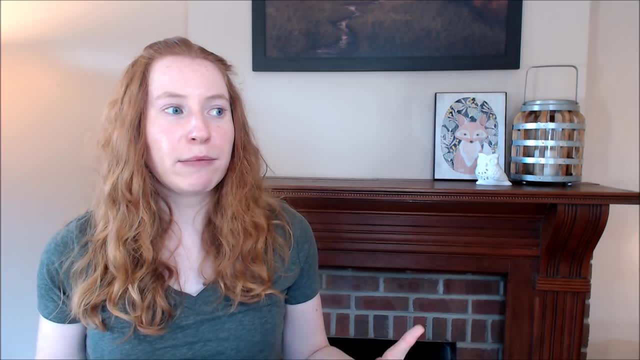 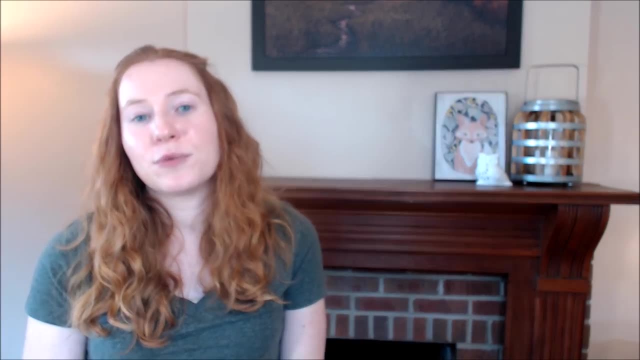 if it's a female character, it will often be that the male characters in the story as a whole are all attracted to the female, And this feels very unrealistic to the reader, because everybody has different tastes. Everybody is looking for reasons to eye on the character. They're most likely to prefer the one that's more favorable. 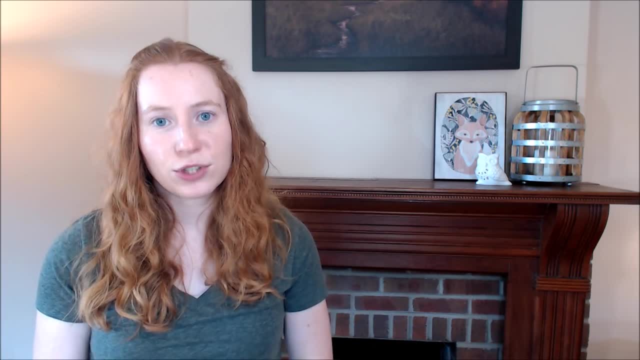 If you like a female character, then you should be more than happy with the male관 in the story. different type of partner and if everybody in the story is attracted to your character, it will not feel realistic. This is very common, It's a. 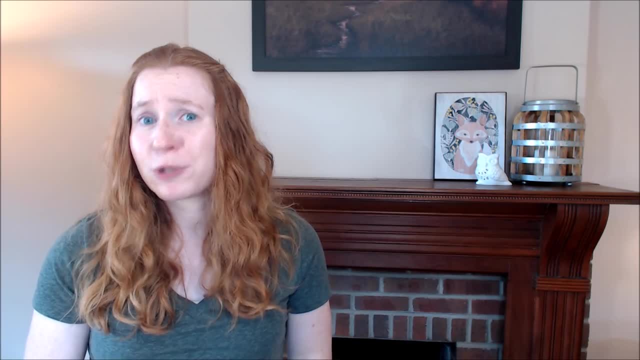 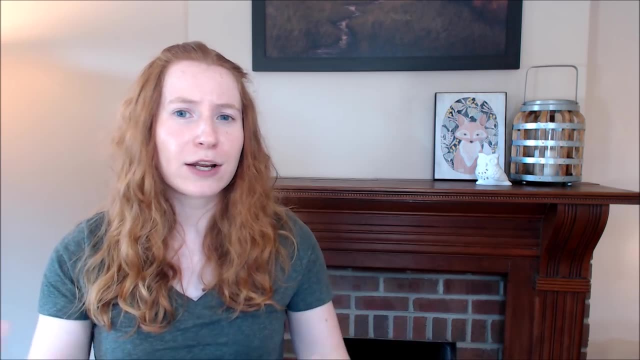 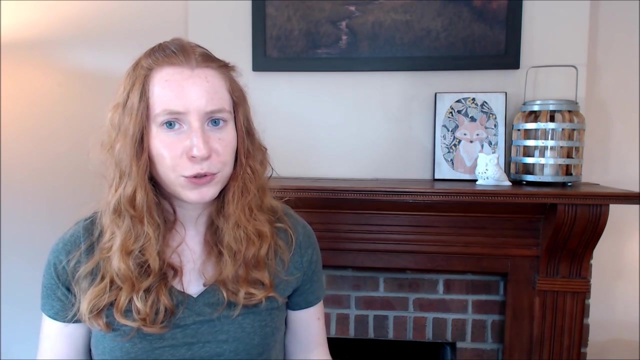 very, very common problem, especially with female protagonists. but it can also occur with male protagonists who have too many women interested in them, just like all the women in the story interested in them at the same time. So I recommend, if this problem applies to you, that you make sure to include characters. 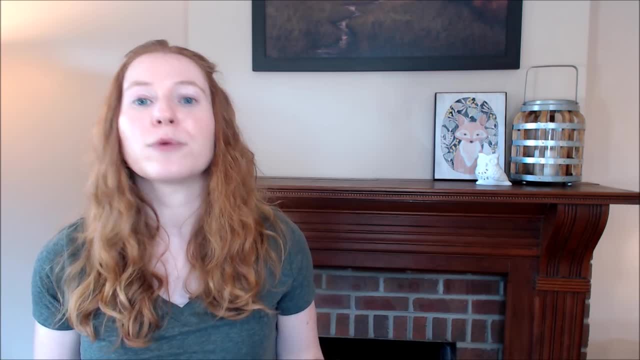 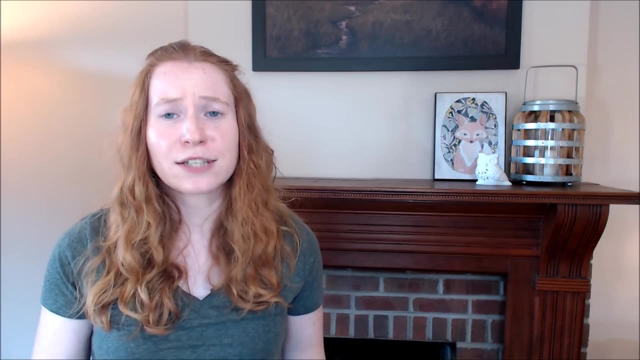 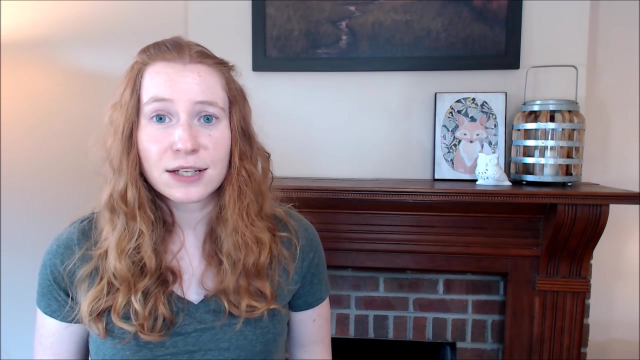 that do not find your protagonist attractive, because that will tremendously help. Obviously, this character doesn't have to say that they don't find your protagonist attractive, but there should be characters of the opposite sex who are not romantically pursuing your character. If everybody wants to be with your character, it will not feel realistic. The next area that 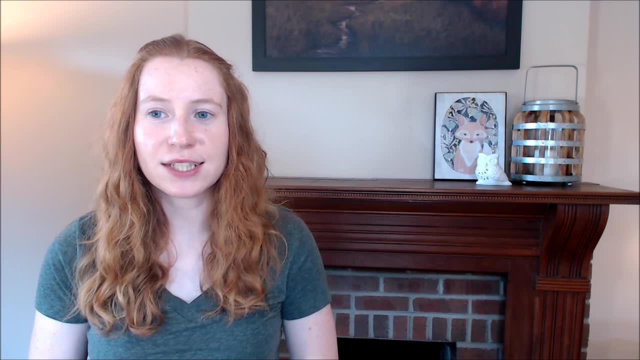 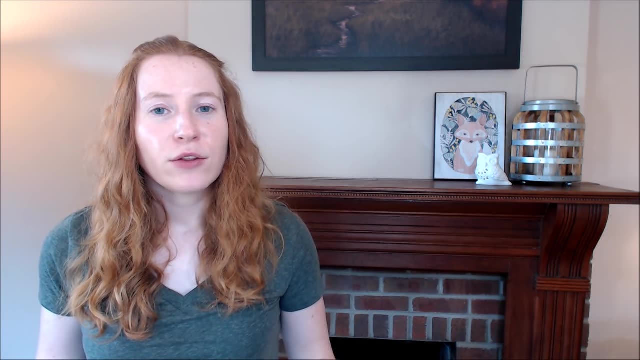 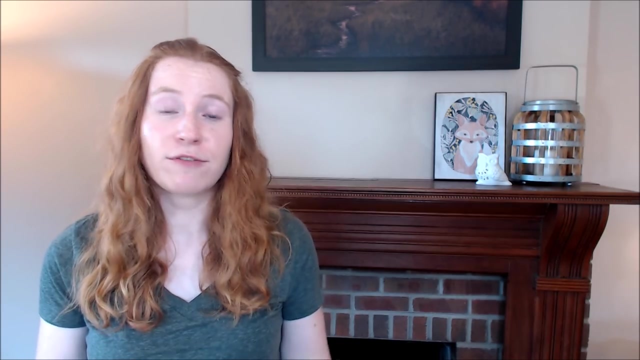 might cause you some trouble with your character becoming unrealistic is if the character has too many skills. If your character seems to be good at everything, that can kind of cause them to seem unrealistic. Most people have a lot of challenges. they aren't good at everything or they aren't good at very many things, and it can be. 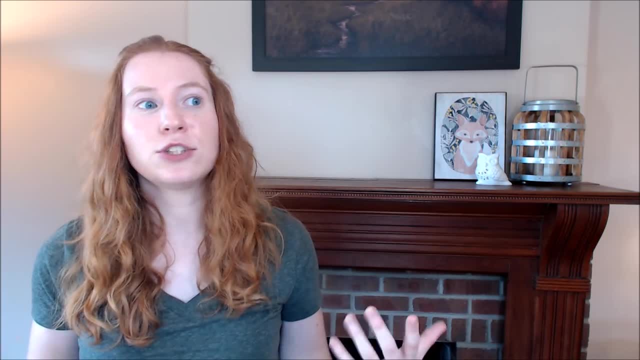 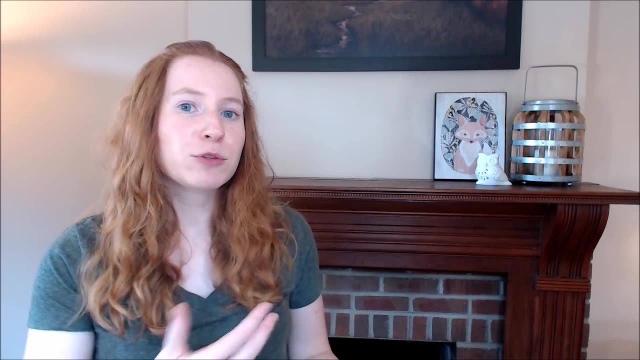 very hard to relate to or really believe a character that's just good at everything. It's much better to give your character a certain area where they're skilled and then have them struggle in other areas and not be completely competent, The other reason you don't want your character to be competent in 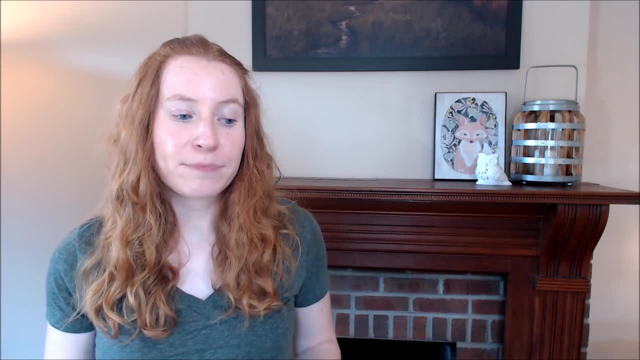 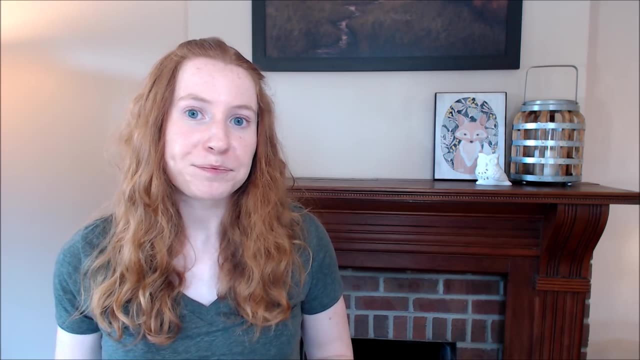 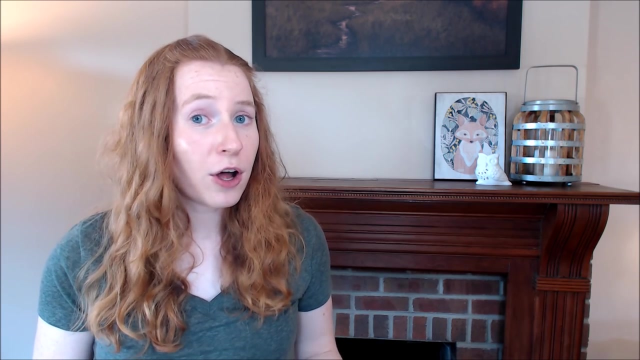 all areas is it just reduces conflict. if your character finds everything very easy to accomplish and very easy to do, There isn't much excitement there in terms of how they solve the problem. Another problem is sort of the opposite situation, where the character actually isn't skilled at all and for some reason everybody turns to that character, or is. 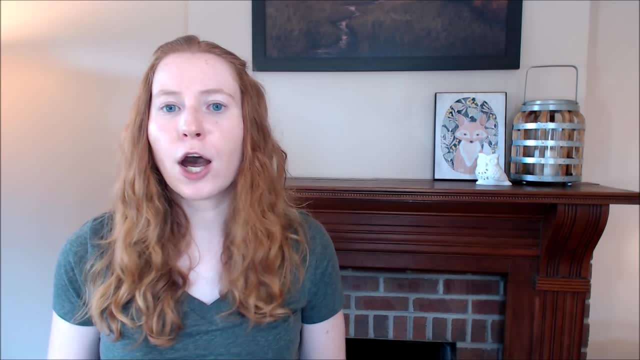 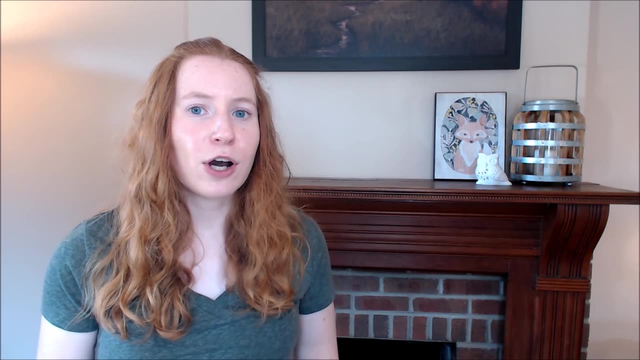 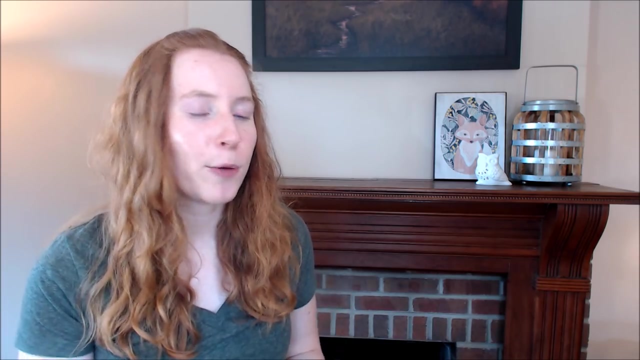 involved in that character for some reason. This is especially common if there is a group of characters with a mutual goal. They may allow the character to sort of tag along with them, even though the protagonist isn't really contributing anything. So this will feel very unrealistic If people are helping. 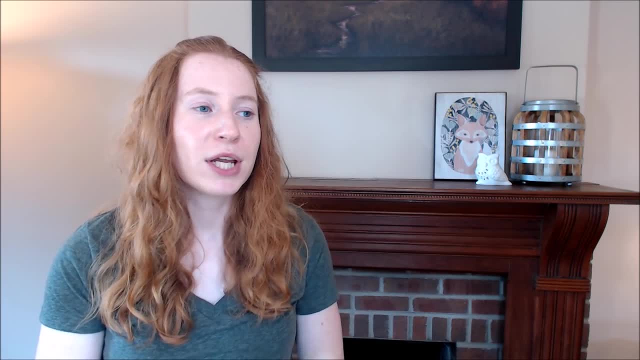 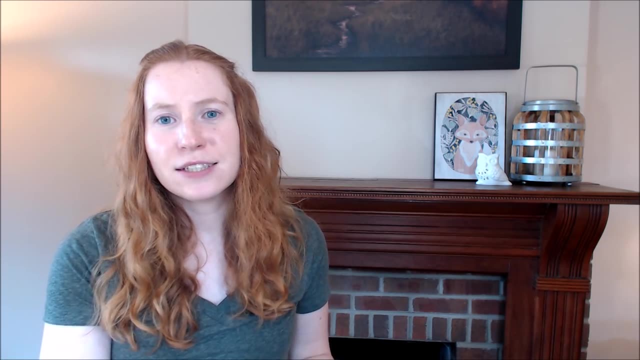 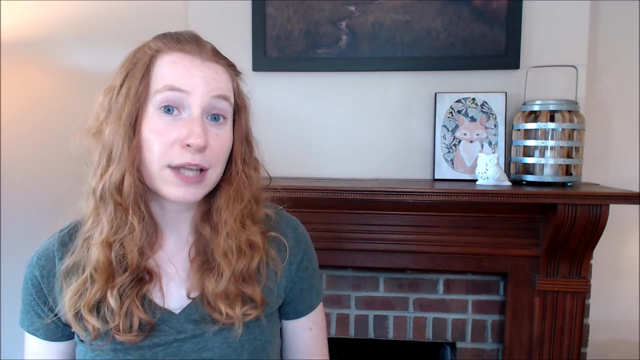 and supporting the protagonist and or bringing them along with the group, but the protagonist isn't contributing anything. that will feel very unrealistic and that's another sort of opposite situation to look out for. Another area where your character could become unrealistic is with their lifestyle. If the character is dating supermodels, lives in a mansion drives. 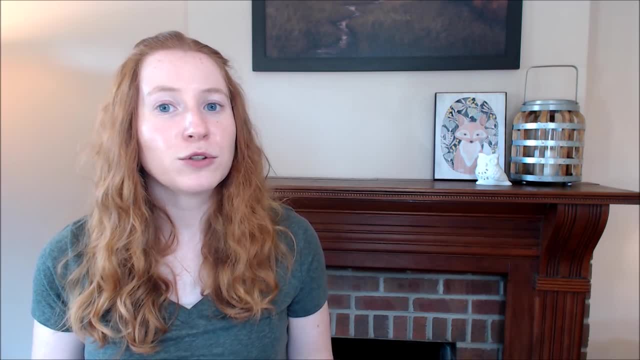 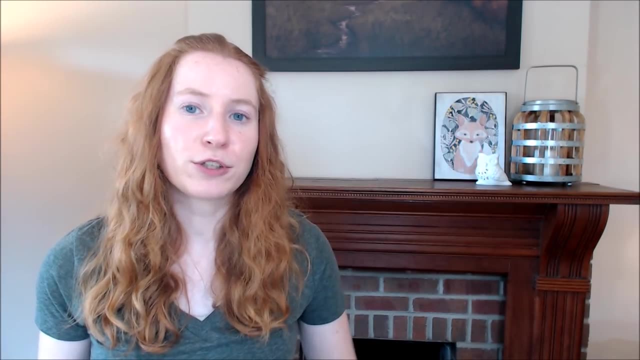 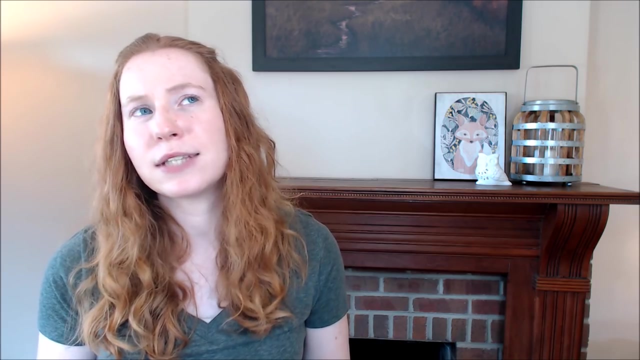 fast cars. it can come across as very unusual, especially if these elements don't have anything to do with the plot. It can feel very unrealistic that the character just has this super extravagant lifestyle. So I recommend not not having that as an element unless it makes sense or unless 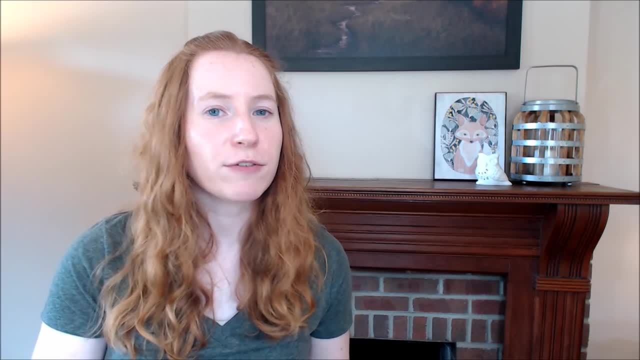 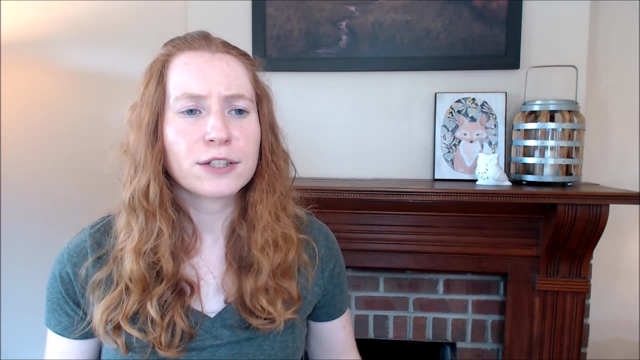 it affects the plot in some way. If it makes it easier or more difficult for the character to achieve whatever they're trying to achieve, then it could become relevant. But if it's not relevant, I would avoid characters who have lifestyles that are idealistic. 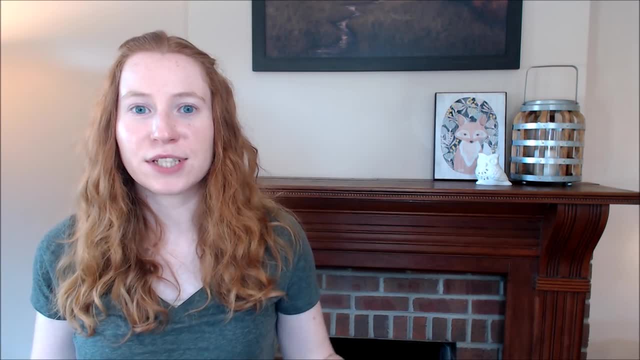 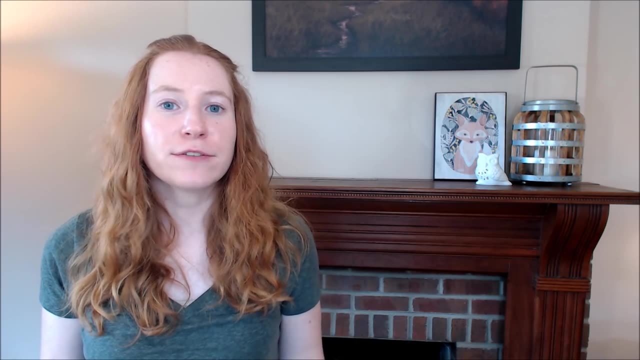 Overall, the most important thing to remember when trying to create a realistic character is that whoever they are needs to make sense, given the way that they were raised, given their lifestyle, given the environment of the novel. It's okay for a character to say: be an expert at magic if they were. 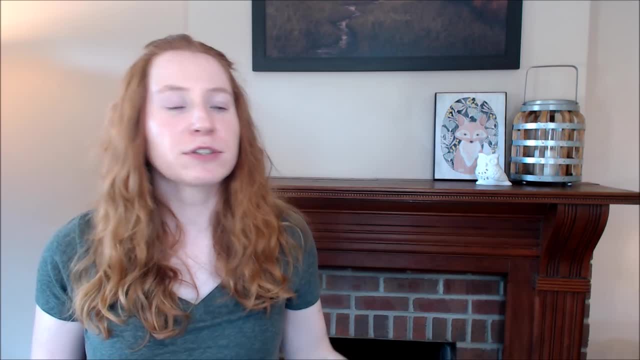 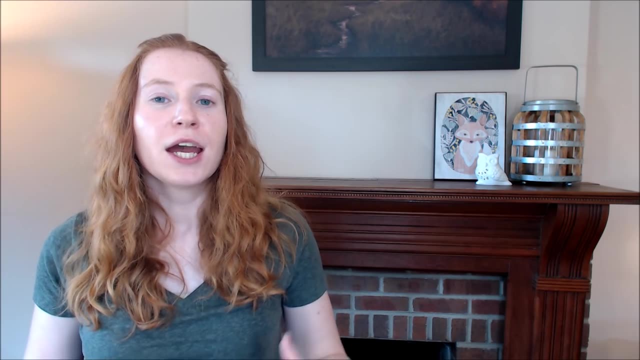 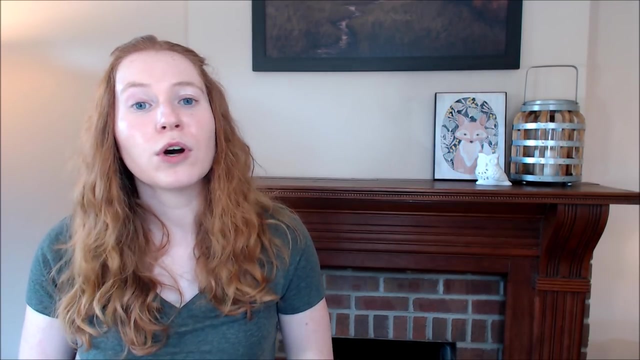 raised to become an expert at magic, but if the character has never seen magic before in their entire life, suddenly develops the ability to flawlessly execute magic, that could come across as unrealistic. It's okay to have the trait, any trait, so long as it makes sense and so long as 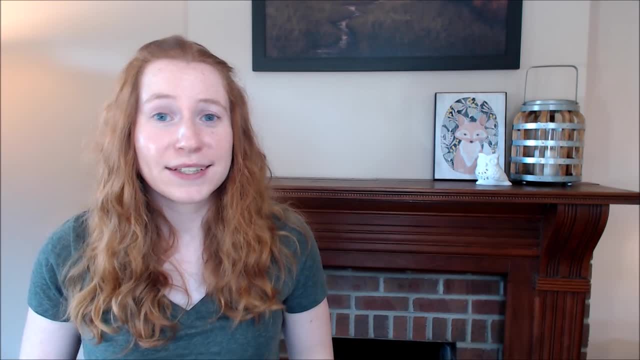 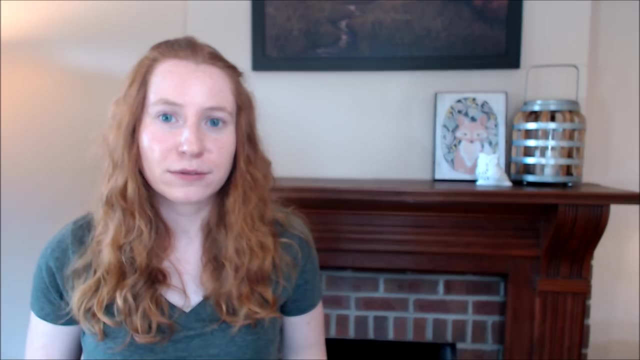 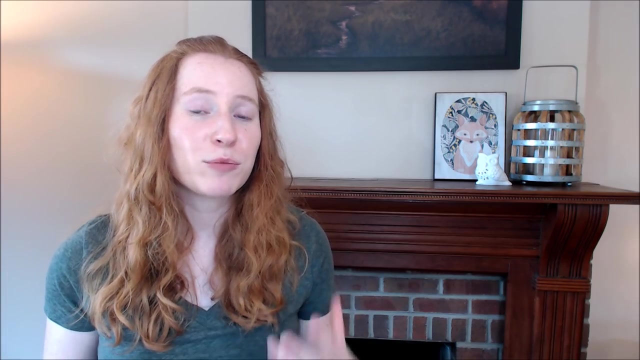 it seems logical within the context of your story. That doesn't necessarily mean that it's logical in reality. it just needs to feel real within the context of your story. So that concludes protagonist week. I really hope you guys have learned a lot and that these tips and this advice helps you to create more. 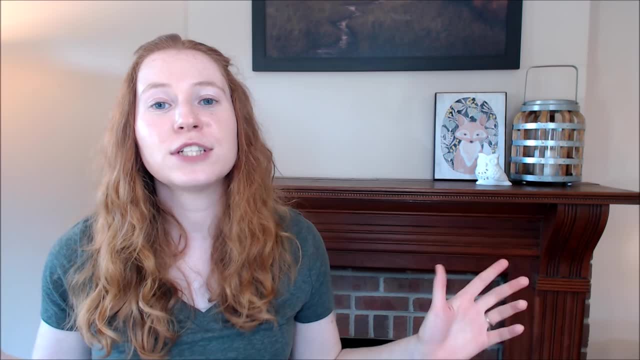 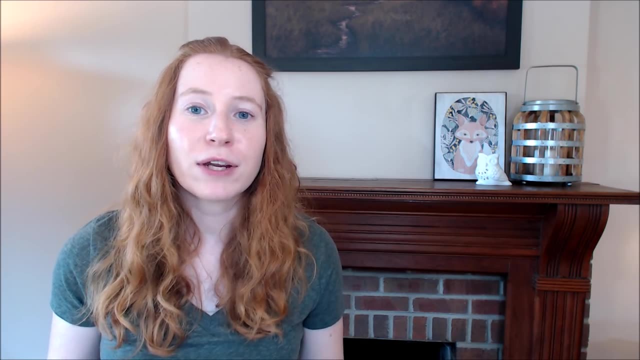 realistic characters, more goal-driven characters and characters that just work better in your story. I hope you'll join me next week because I'll be going over plot structure and it'll be very helpful. It'll really solidify a lot of the ideas we talked. 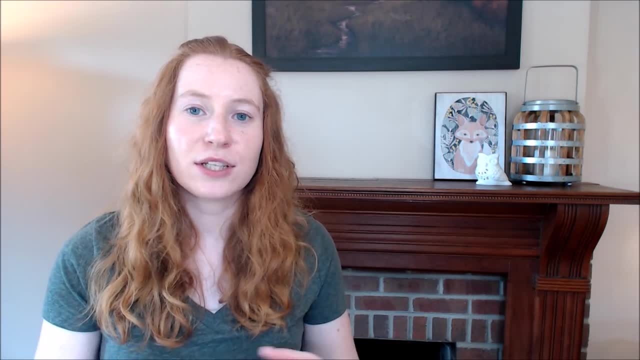 about this week. It'll help you learn how to apply those things in the overall structure of your novel.